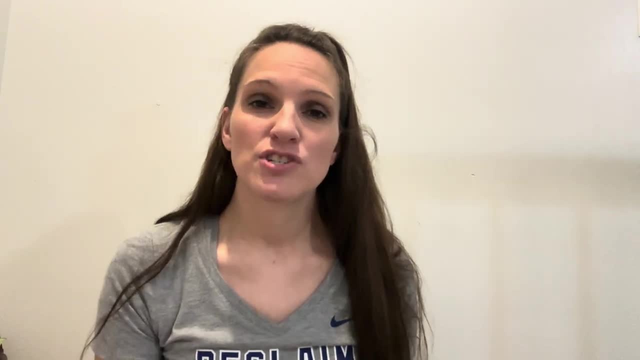 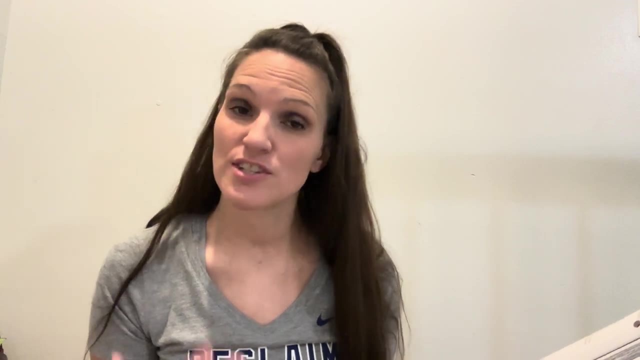 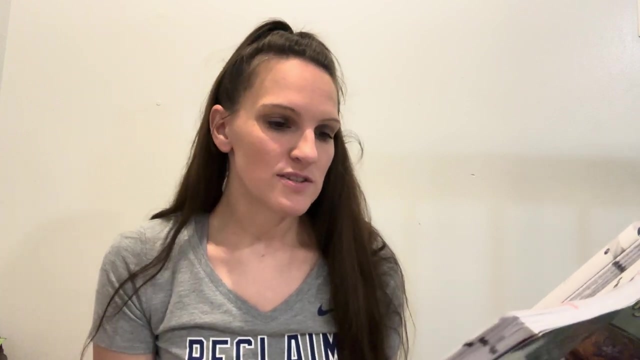 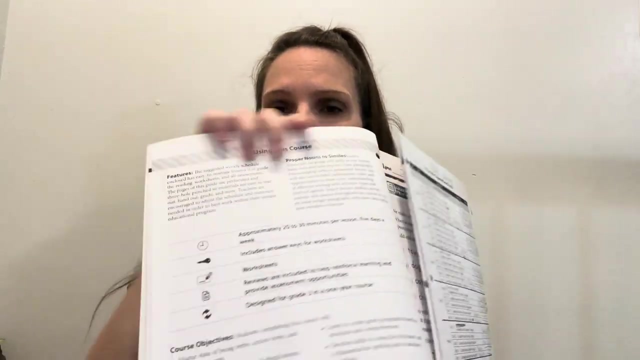 grade number 3.. And then, as I have shared previously in other videos, one of the main things that I really love about Masterbooks- besides it being a good Christian curriculum, this is a Christian curriculum. It goes over a lot of scripture and things throughout and puts a lot of biblical things through it, So I love that. But also, as they have the schedule laid out for you at the very beginning of the book, this is a five day work. It'll say what it is, It's for five days and then it'll have a schedule wrote out for you. 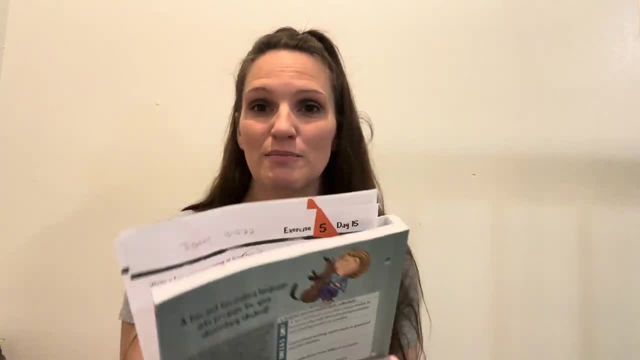 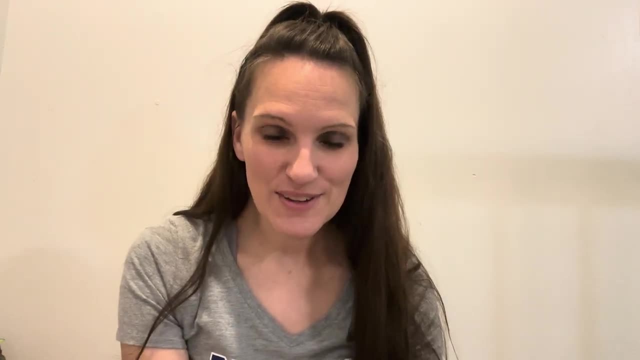 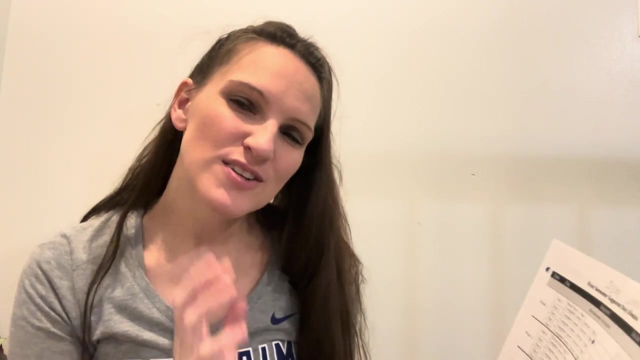 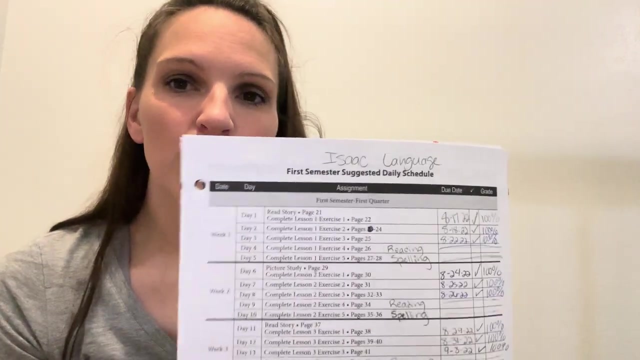 So I'm just going to try to hold on to what I can and show you guys and go through that. So I will say a couple things that I don't care so much about. but I do love this curriculum. It is a good curriculum. I love Masterbooks, So it'll have your week. This is grade 3. as I said, This is kind of our schedule. 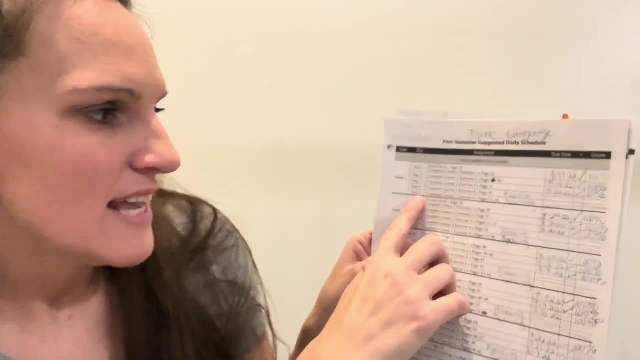 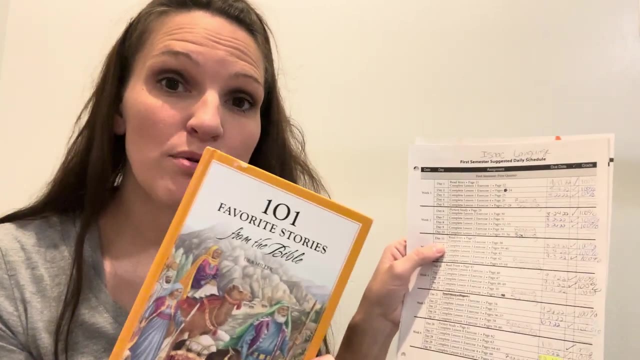 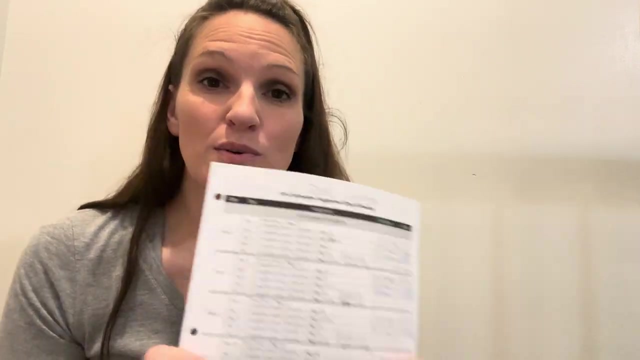 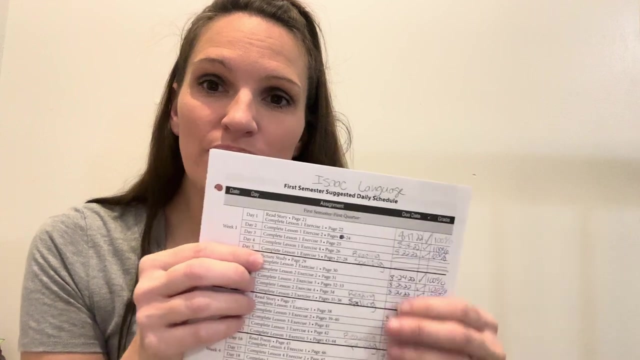 So you can tell day 4 and day 5 every single week. Day 4 will be your day that you do your reading, which is their Bible, And day 5 will be spelling. So what I decided to do, after about three years of doing Masterbooks, is I wanted to hit hard on the reading and the spelling, So I took those two days and I marked them out for language, And I use this as one day of reading. 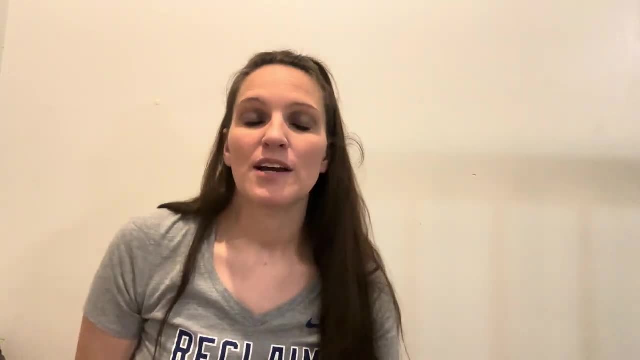 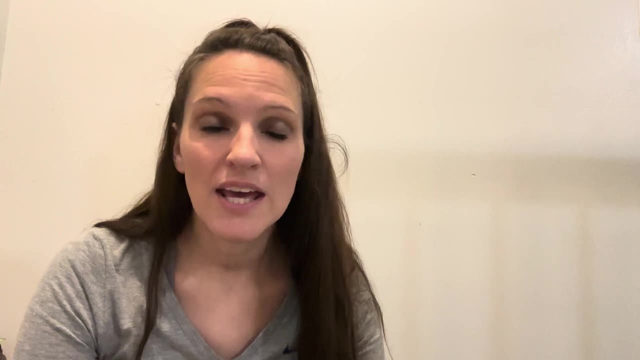 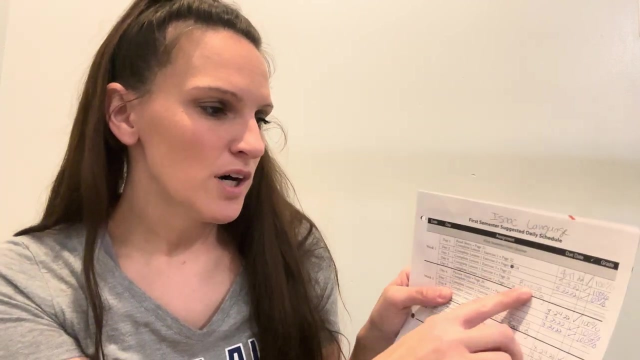 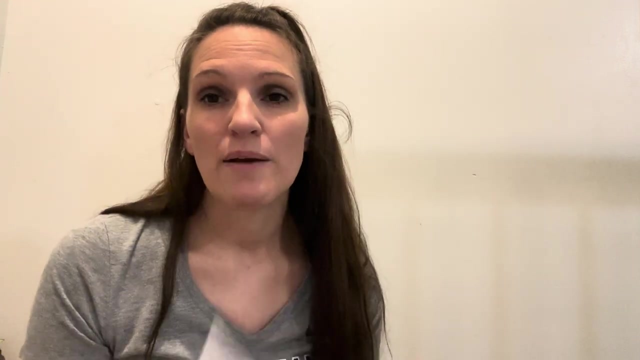 And then the rest day of the week. we went to the library one day a week and we got books And I had them read whatever books that they picked for so long- 20 minutes a day, And that way it could be more reading. I felt like they wasn't getting enough reading. So day 4, that would be one of their days that I chose. It would be the first day of the week on a Monday That would be separate from language, So I pulled out all the language reading for that day, day 4,, which was this: 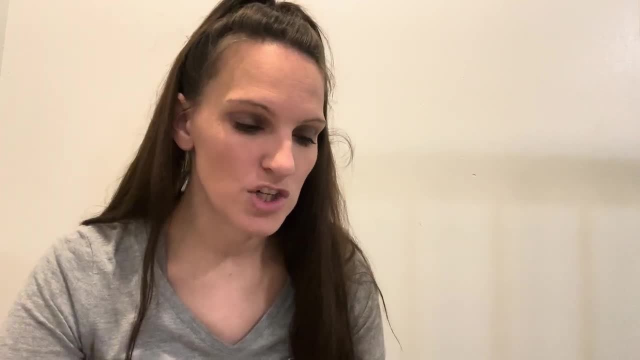 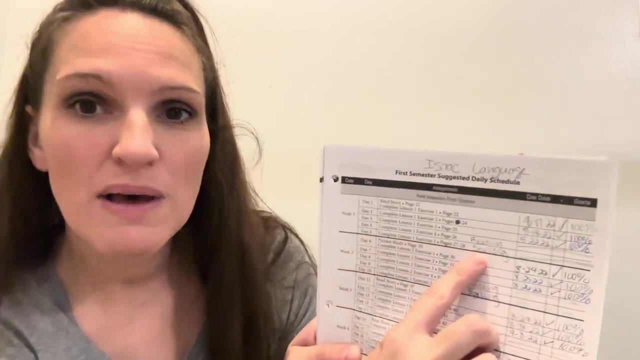 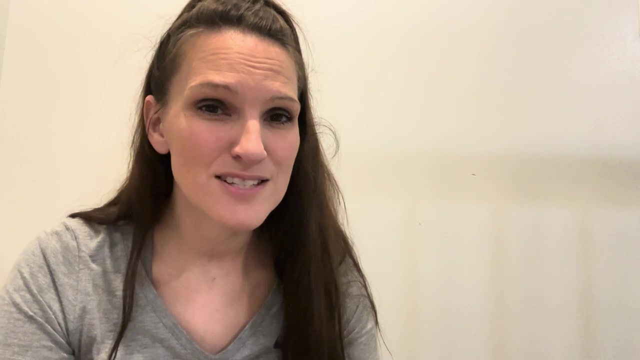 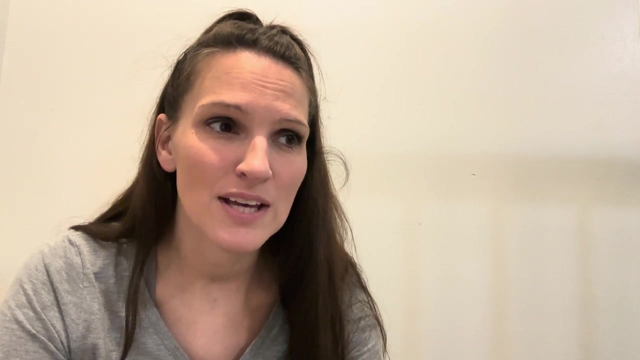 And then the rest of the week they're reading 20 minutes a day, whatever book they chose, And then every day on the fifth day- not every day, but every week- on the fifth day was the spelling. So and the thing that I didn't like about that is that's the only day they had spelling And that was the last day of the week, And they gave your spelling words for the last day of the week. So that kind of was just like: okay, they do have a list at the back of the book of all the words. 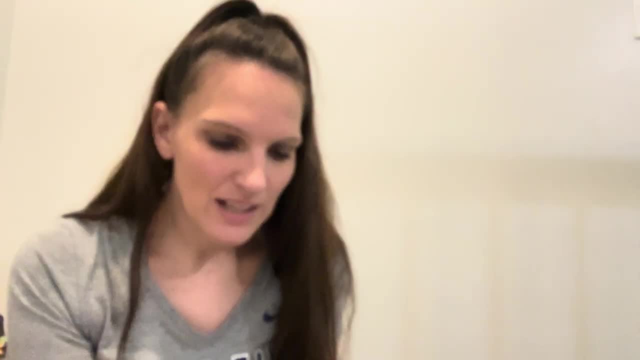 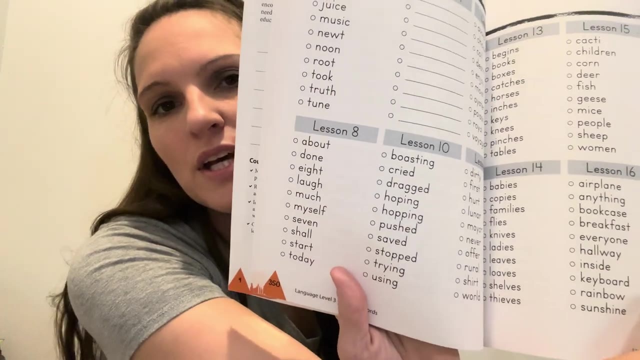 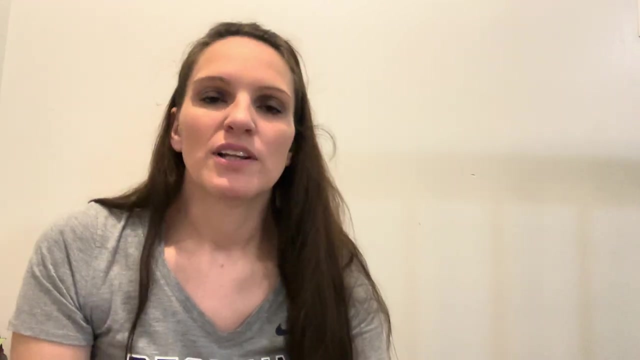 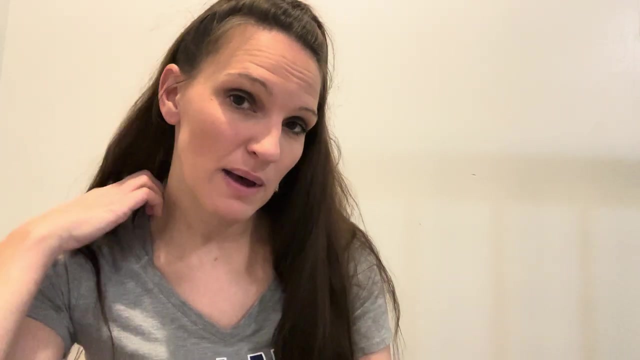 So you can pull them out. So you'll have, like, your spelling words at the back of the book You can pull out. if the kid likes to maybe hold on to it, You can cut out or whatever you would like. So that was nice, to have all the lists together in the back, all the words together. So what I did is I took day 5 of spelling. I would give those that page So like okay, so look, this is a day 5.. 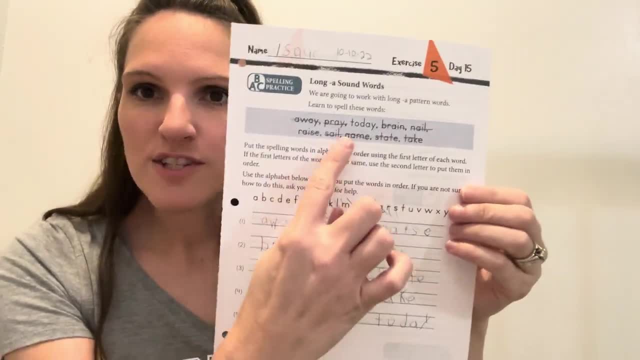 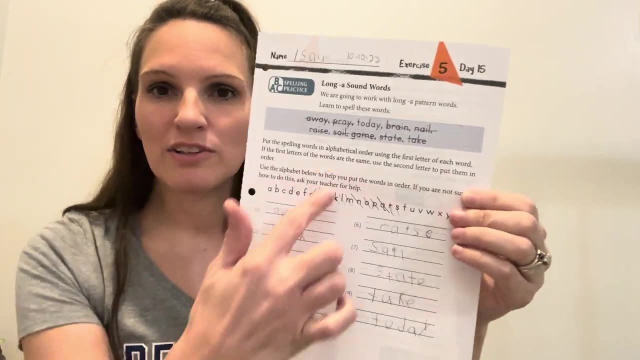 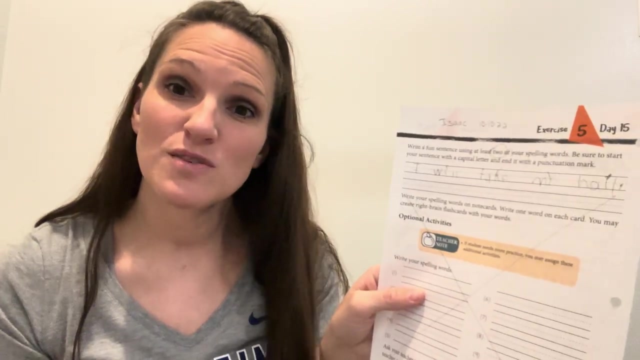 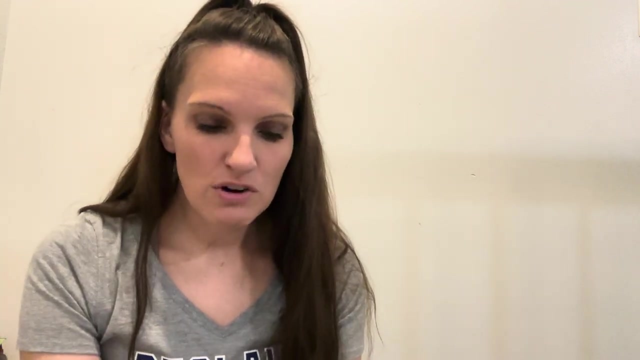 Of the week. they're spelling words right here. So I would take this page and I'd give it, rip it out and give it to them on day one. That way, Monday they would get their words and they'll have a little bit to do fretting back. usually Here is extra work for writing, but I marked that part out because what I did the rest of the week is I had them say spell right, say, spell right. say say spell right. Okay, say the word. you're going to write it, you're going to say it as you write it, which really got old. Honestly. we've been doing that for a while. 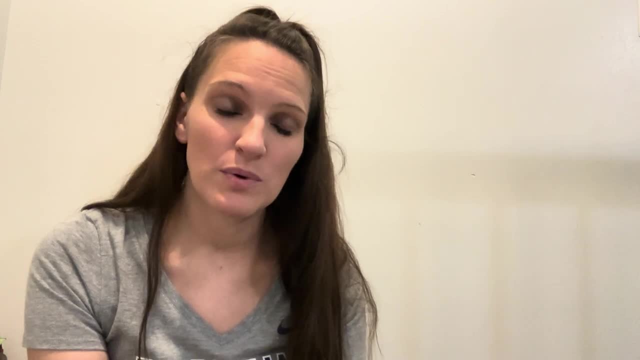 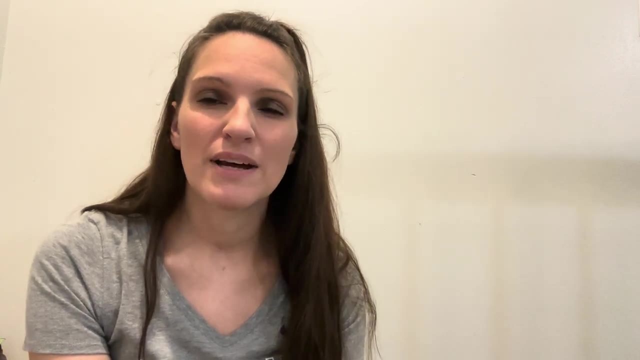 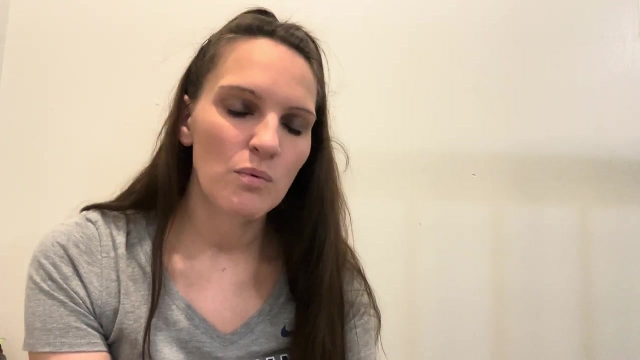 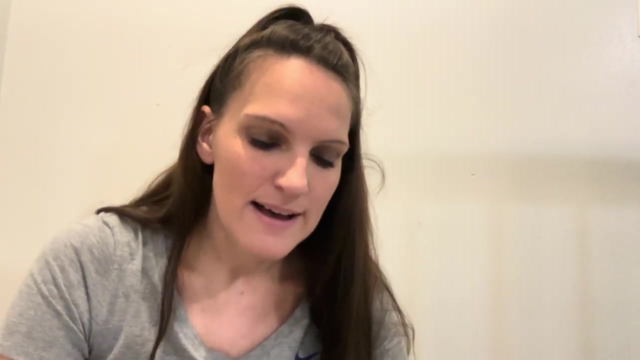 Which is a reasoning why this year we are not doing master books language. It is good And maybe it fits for people- you know may fit for different people- But it just wasn't working good for us. It wasn't a good fit for us. We did it for several years. We did like it. We like that. it wasn't too much of an overload. But also I feel like we needed more. We needed more with the reading, We needed more with the spelling, And so that's what we elected to do, So let's get more into it. So you've seen the schedule. 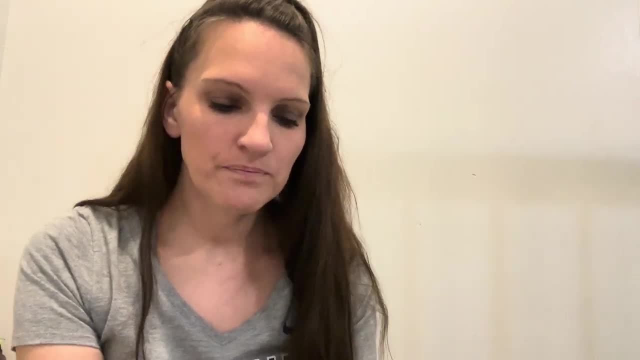 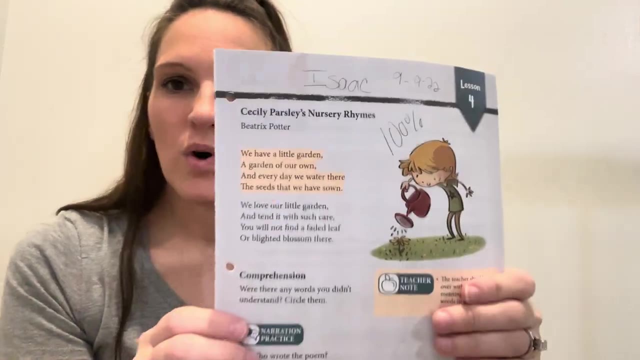 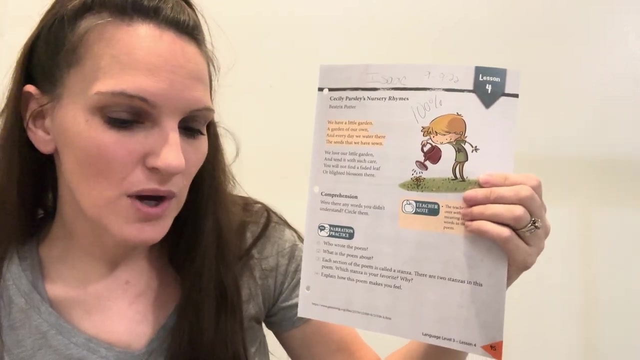 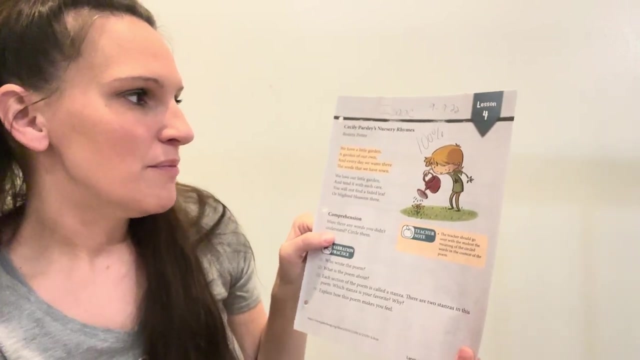 And what I kind of did, So usually on day one, so I pulled some of these pages out loose in there. So so, like day one, usually you will always have- And this is also for the next grade, level two, which is well fourth grade and fifth grade- you will always- usually see, on day one you will usually have a word, picture or a poem and you'll have a few questions. A lot of times I'll have a few questions. 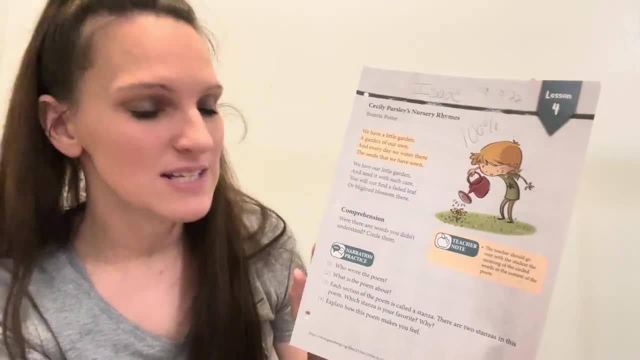 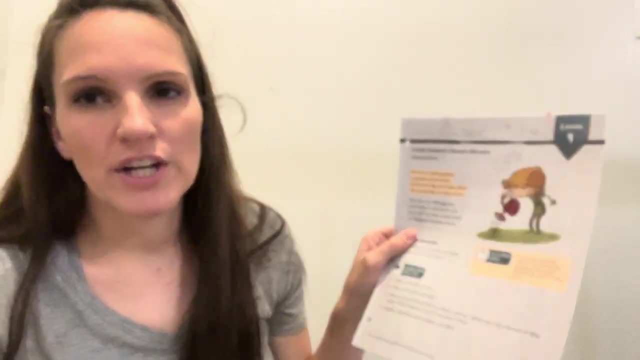 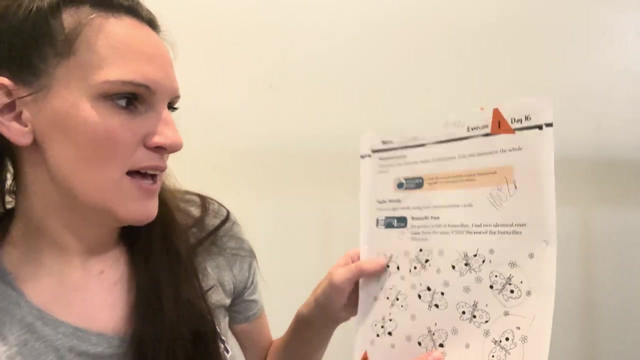 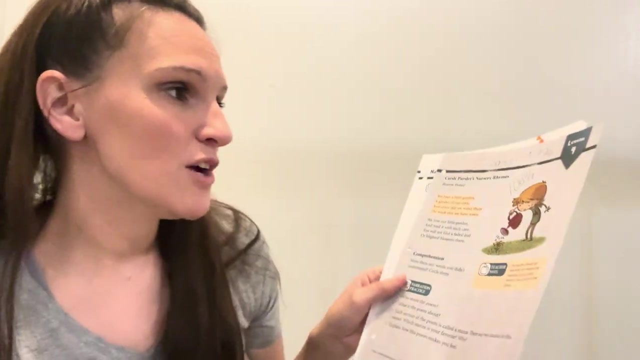 I just had my kids go over that with me. That's something we did together. That way they can answer these orally. They don't leave a lot of room to write out your answers there Sometimes. I just said: just write your answer, I'll look over it later. So anyways, they would have that for the first day, just kind of open up the week and something else. Whatever it is, it's never really the same, but then you always have a poem or a picture study on the very first day. So day one that's usually what you get date to. You'll go over whatever studies it is. So if it's pronouns, 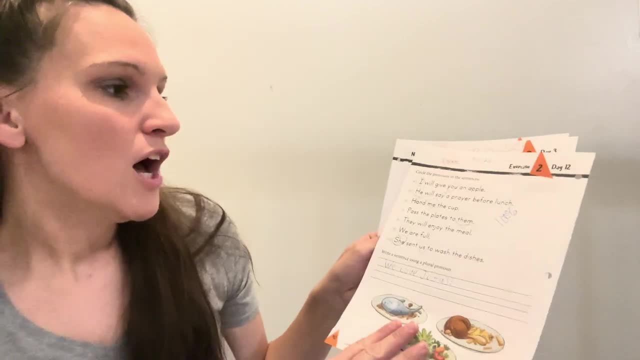 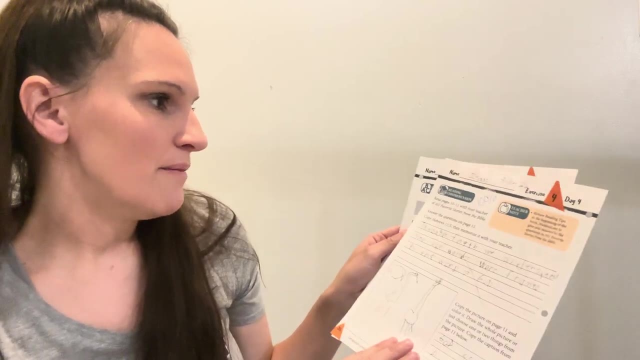 or verbs or whatever it is. you'll go over those. It's usually two pages a day, So this is day two. you have front and back Day three. you got front. Okay, You got one page this day, So this day you. 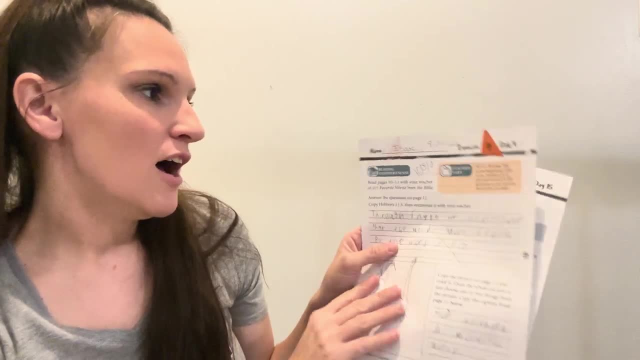 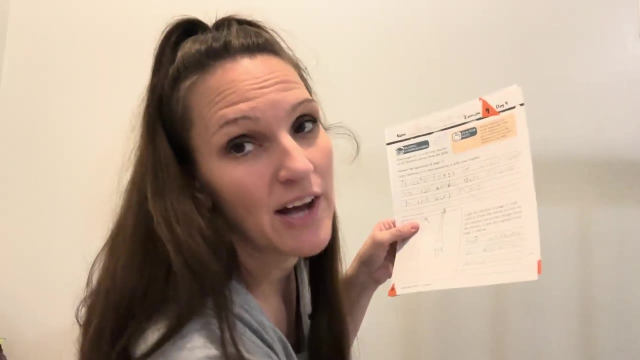 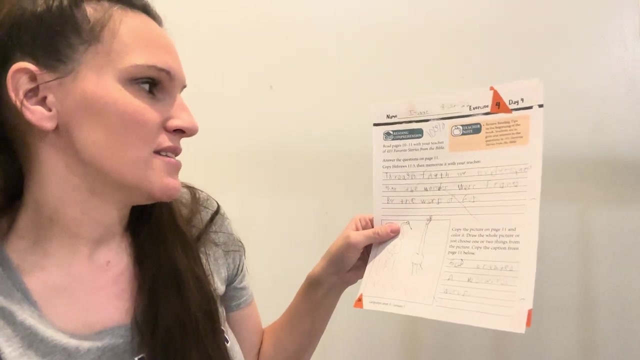 only had one page And then on day four, as I said, is the Bible book. So you will. you would need to get out your this here that you would need to buy with it. It comes with it, but you need to make sure and click it and put it in your cart. So it would basically say: read pages, blah. 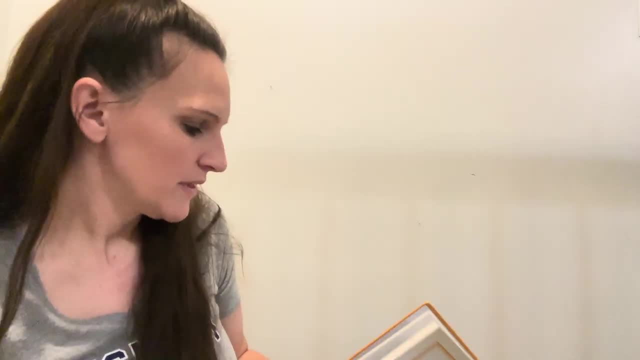 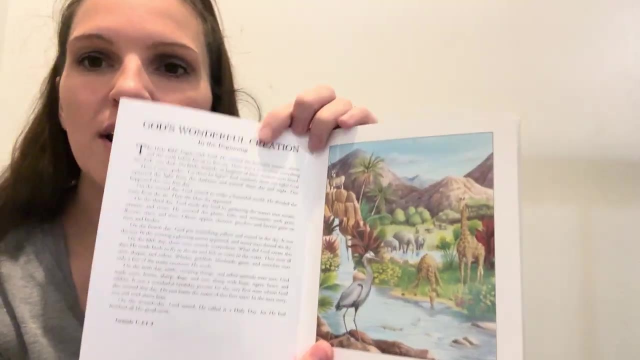 blah, blah in your book. So you would go to that. So let's see here: read pages 10 and 11. So you would go to 10 and 11. So you'd read the story right here. It's not too bad. And then you got. 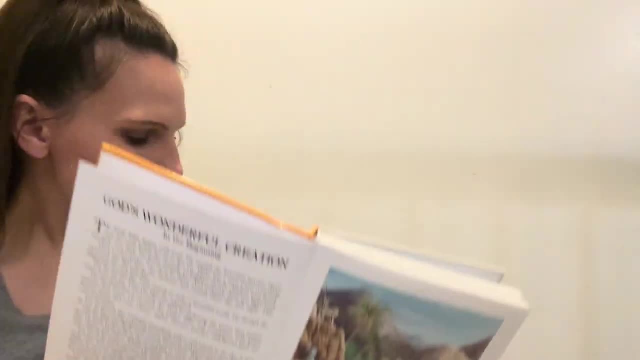 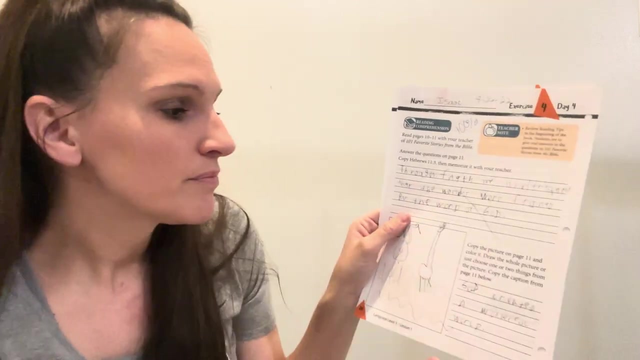 a picture study over here with questions. You would have to answer the questions. Then you would take this and it'll tell you: this is all about. you're going to fill out about this page, So you would need to copy the scripture. Then you would need to copy what the picture was about: copy. 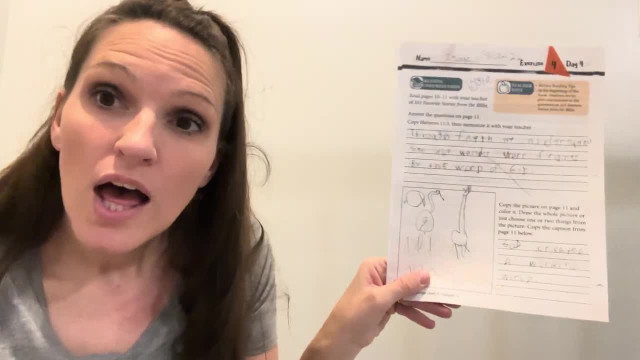 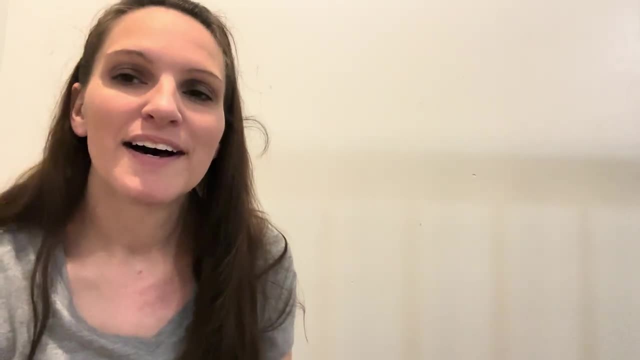 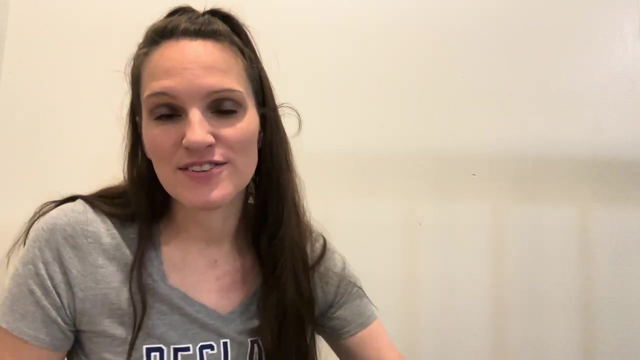 whatever the picture was about. Then they have you draw the picture, something similar to whatever it is. Um, my kids, um, at first, um, as I said, we've been doing masterworks for a few years now, So, um, this just got as they got older. they didn't want to be drawing pictures and they just 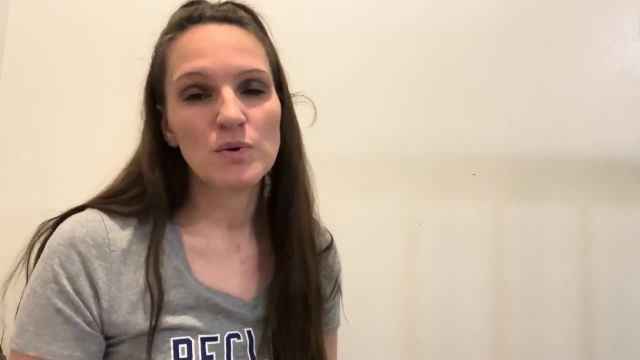 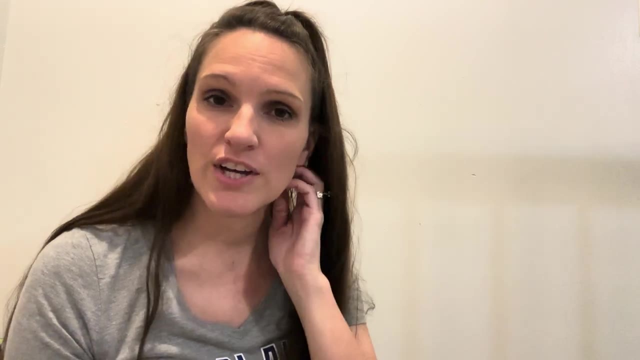 didn't want to be copying out of scripture, which sometimes I may have them do it after a while. Um, I just had them read the story. They were getting there with some reading in and answering the questions and make sure they comprehend. So 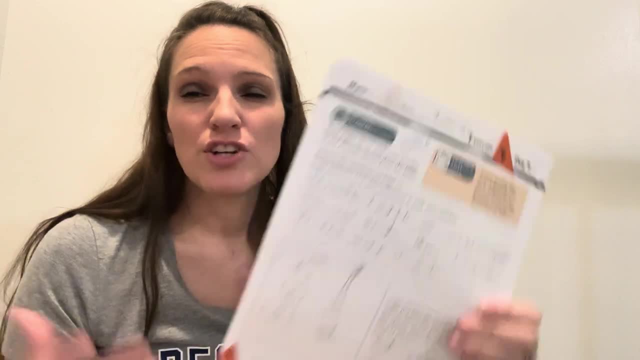 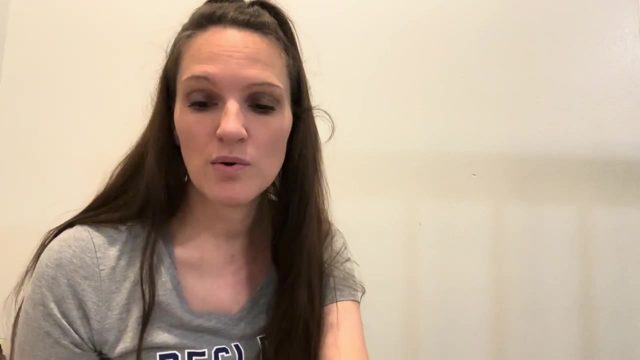 sometimes I didn't have them draw the picture or whatever. You just got to do what's best fits for your family. Um, so that's the great thing about homeschooling is you do what's best for you and what works best. So if your kid is not very thrilled about I, don't really want to draw. 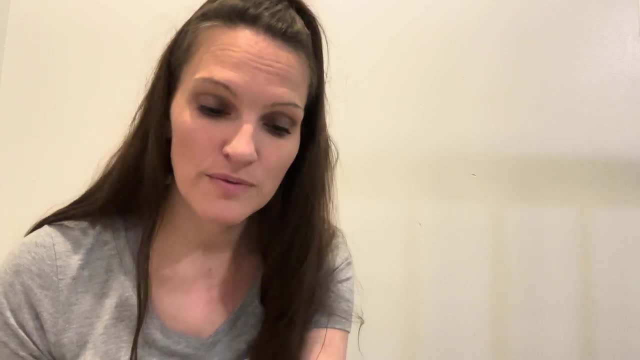 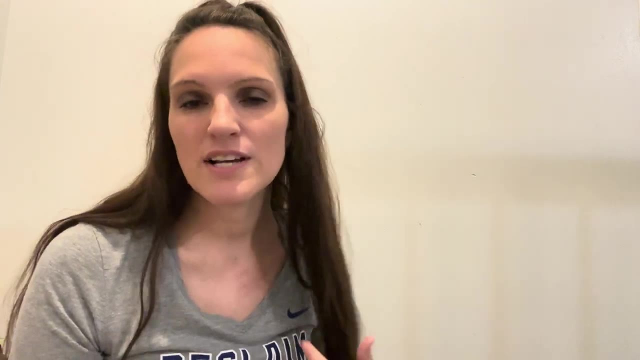 this picture today because I know I'm getting sick and tired of drawing copy and whatever picture this is. you know, cut that out and do something more. do reading, more reading or whatever it is. So that's kind of what we did, But so that's kind of. look at day four: every fourth day. 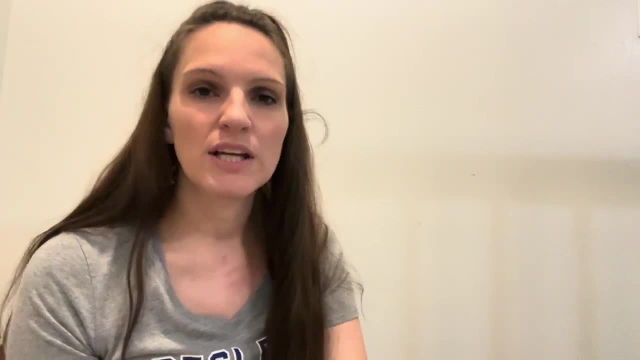 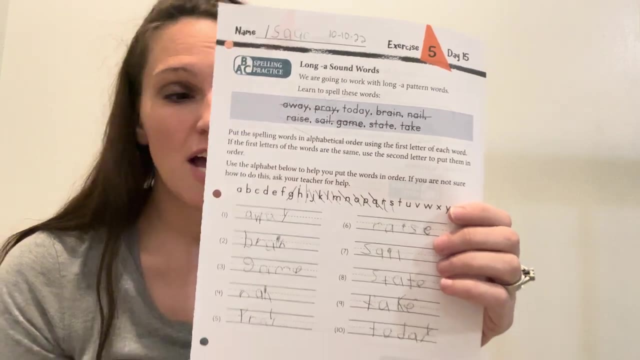 you will be your day for your um, your Bible, reading that as I talked about in that book, and then every day five, as I shared, you will get your spelling. So this is what a day five looks like: front and back. Sometimes they'll say extra optional: write your words too. 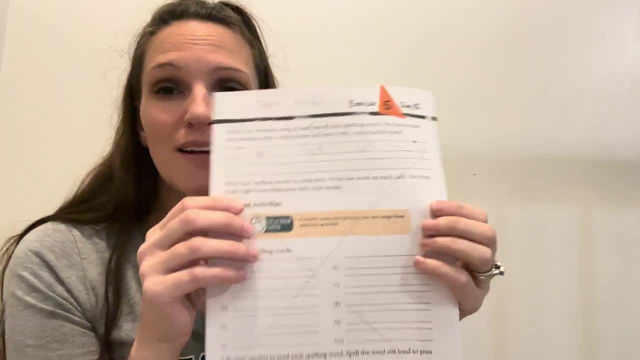 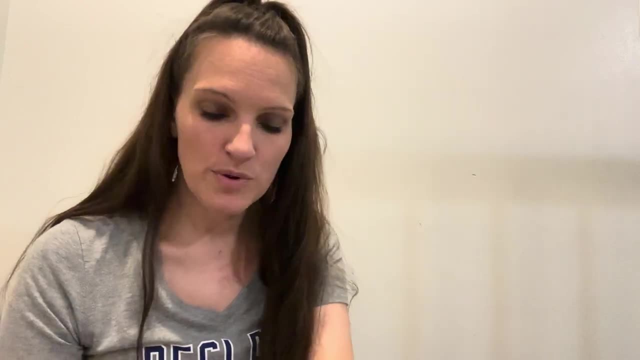 So we'll give you it, ask a few questions And then, um, you can write your words or whatever extra, which my kids already were writing their words, uh, three times every day saying it. so i didn't want to add on for the monday that i did choose. 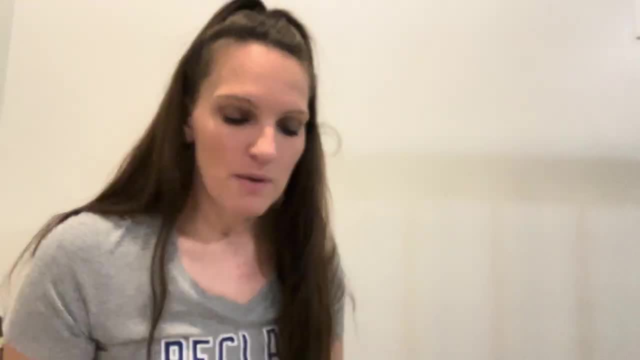 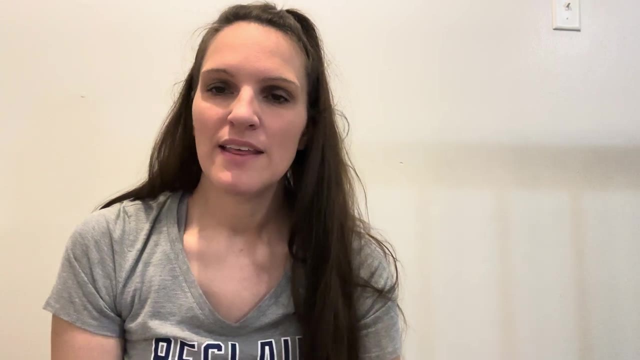 to give them this page. i didn't want to add on extra writing that day, so that's why that was marked off. day five: um. that ends the week with your spelling, and then um. it's just basically the similar. throughout the rest you'll just go over different things, but day one will always. 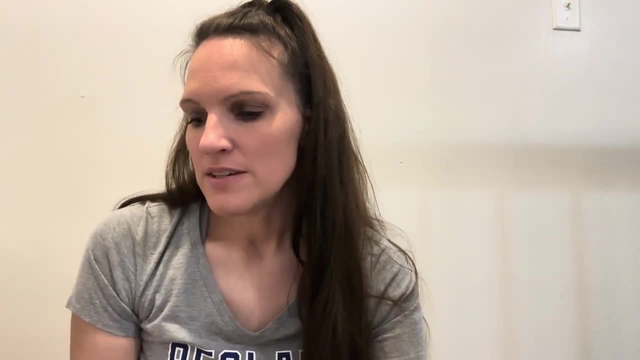 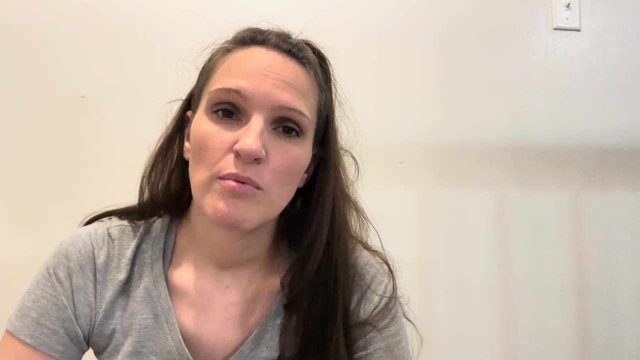 be the picture, study or poems, and then day two and three you'll have your work going over, uh, different language things, and then day four will be your reading with your bible, day five, your spelling. so, um, you can pull those out and do whatever you would like to do with them, they do. 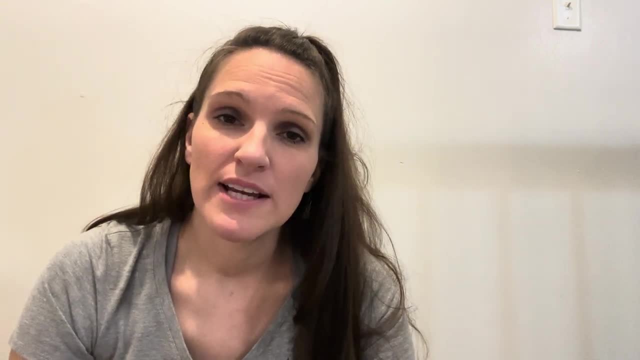 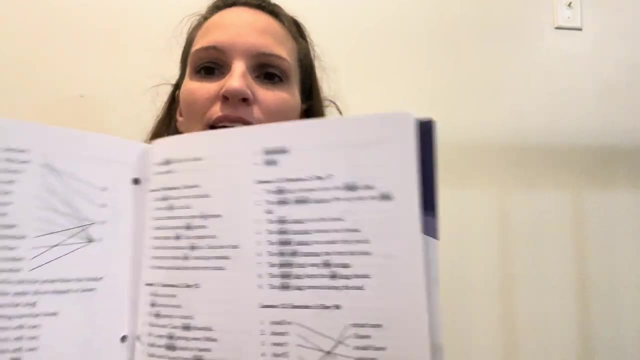 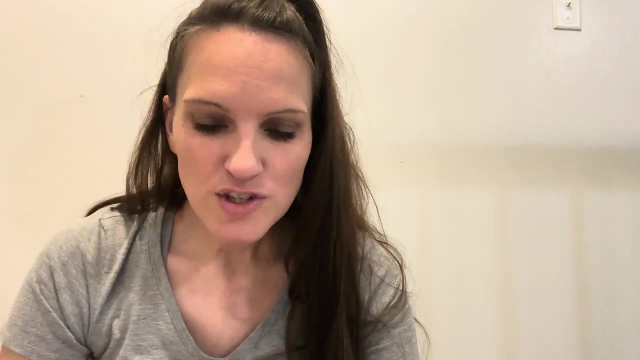 have your um your lesson plans laid out in the beginning of the book, which i really liked, um, which was awesome, and then in the back of the book. you will always have all your answer key to every single question and problem comes in the same book. so that's really really neat. um, masterbooks was real good. um i just this year. we just wanted to. 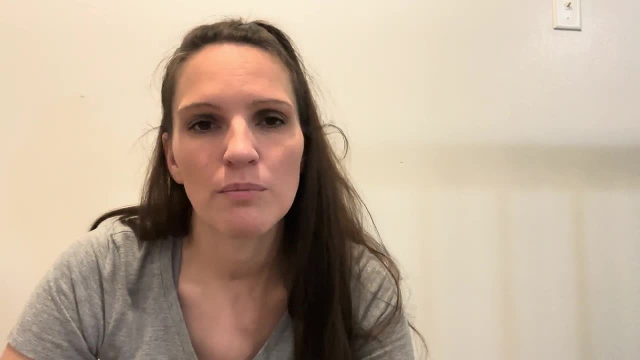 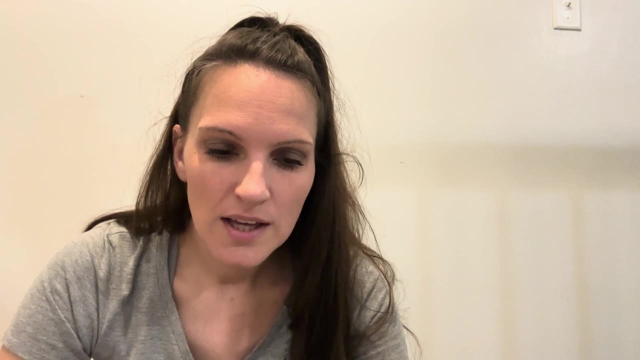 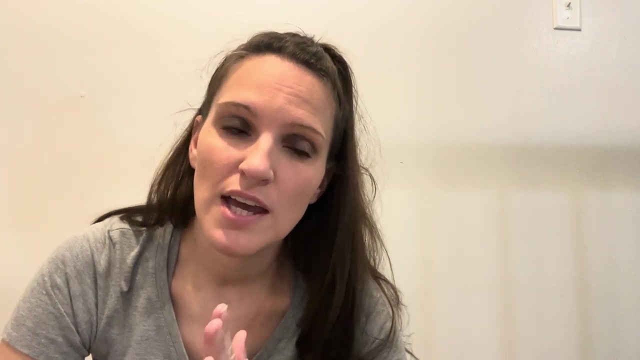 change it up. um, since we kind of had to pull out the reading, we kind of had to pull the spelling, i just wanted to do something different. um, so this year we are doing um spectrum, we are doing a spectrum reading. it's a whole entire year of reading, every single day. um it goes, gives them. 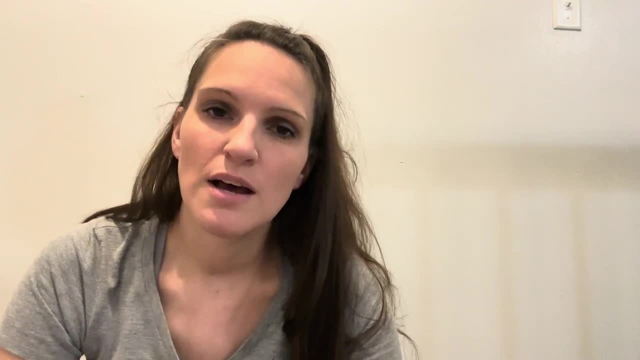 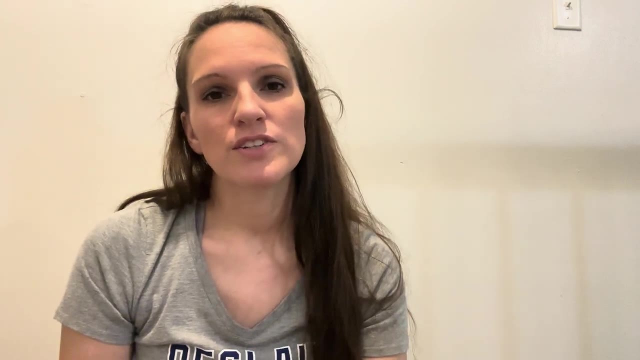 something to read and you got to answer questions for comprehension study, um. so i like that. and then we are doing spelling of spectrum also. they give you um page every single day and at the end of the week you will have um, your spelling test. so i really like that. i like how that's laid out. 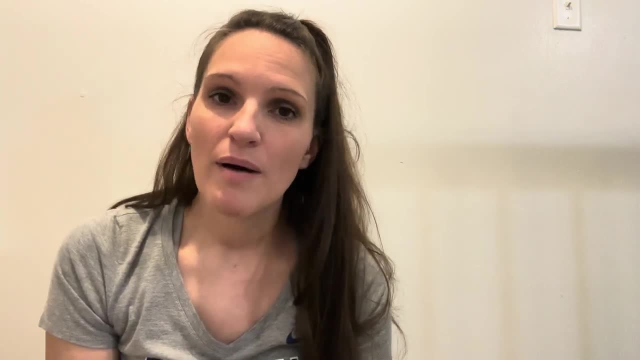 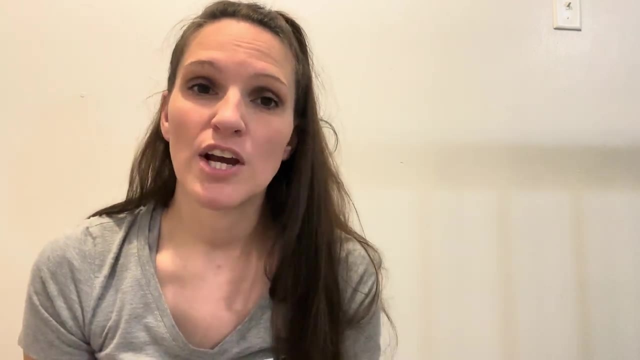 and versus having one day for reading a bible story and then one day they only had for spelling, which you can- yeah, you can have your kids write spelling words every day or whatever else you may do, but i liked how it was actual book and every single day it, you know, has something read out. so 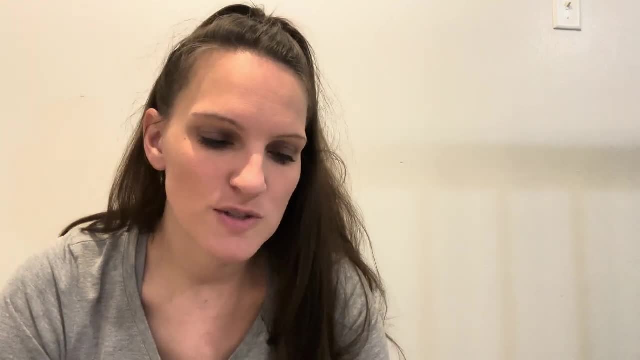 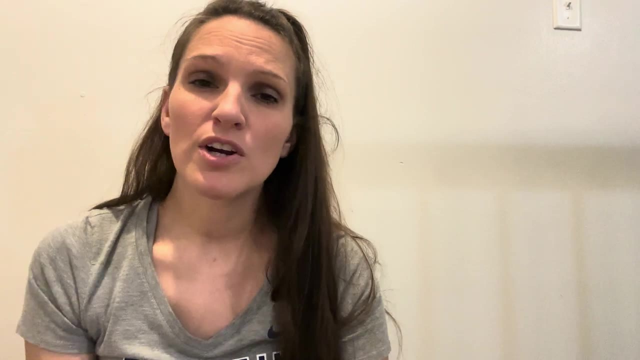 it's a great way to do that. and then we also did language um, something else, and then we also did spectrum the language. so we have three different, separate deals. we got language, spelling and reading um, and then we are doing also a cursive, um, my girls have taken cursive. i think it was a. 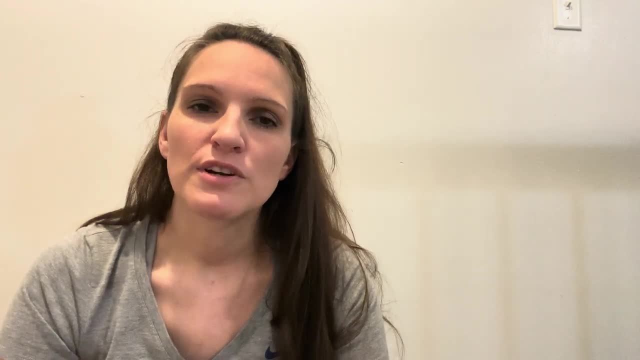 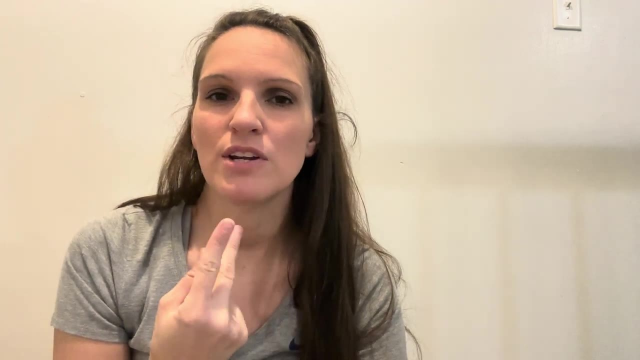 couple years ago, but we are doing another course for them, um to refresh their memory. and then my son is learning cursive this year, so he'll have his own writing. so we have four different things. we get reading, writing, spelling and then language. so four different things. so we're going to talk a. 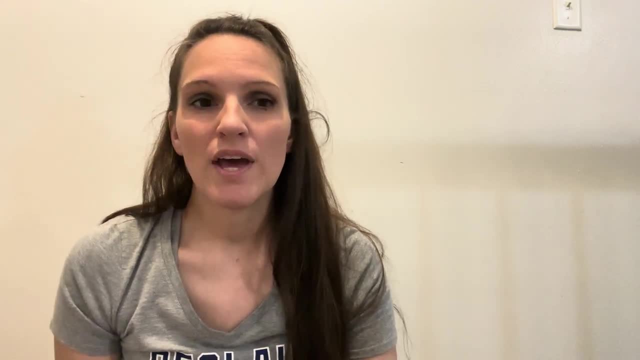 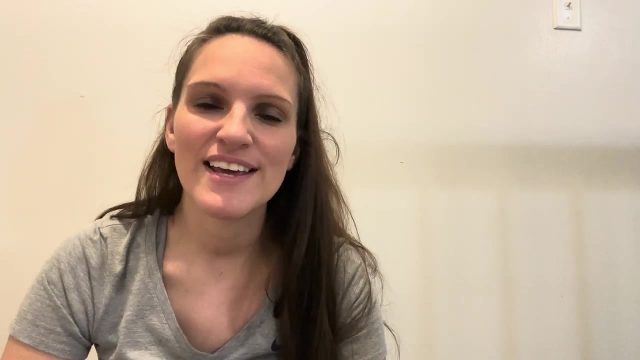 little bit more about that in a little bit more detail in a little bit more detail in the book. so they're getting a lot more. i feel like doing it this way: um, i'll do a review on those. videos are on those curriculum spectrum and kind of give you guys an idea how that is and how that's going. 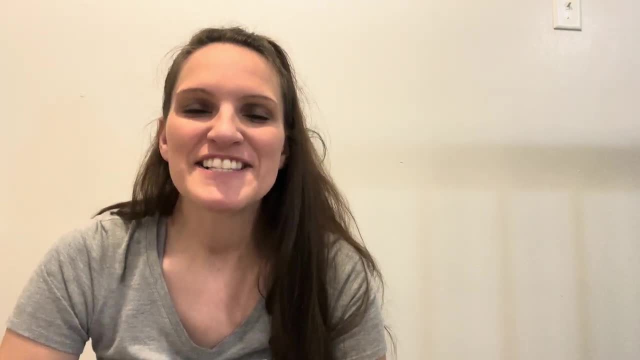 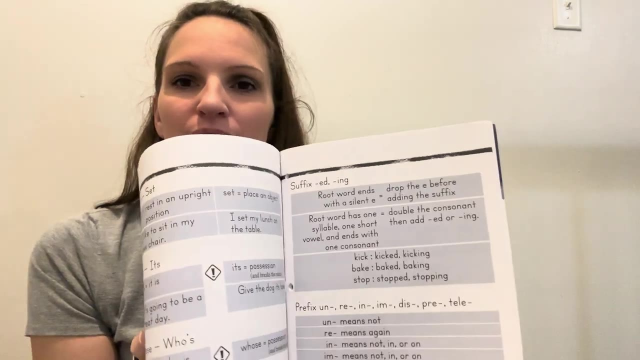 um, so far, so good. we're, i think about what- about a month into school year now? so it's going good so far, um, so that is kind of the sum up of this. um, they have other things in the back, um studying pages, um things that you could rip out. a lot of times we would rip those out and put them in a. 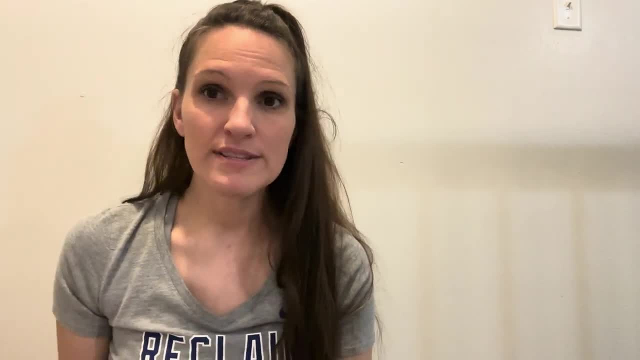 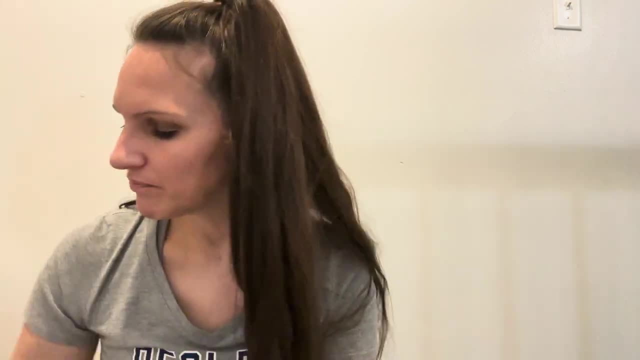 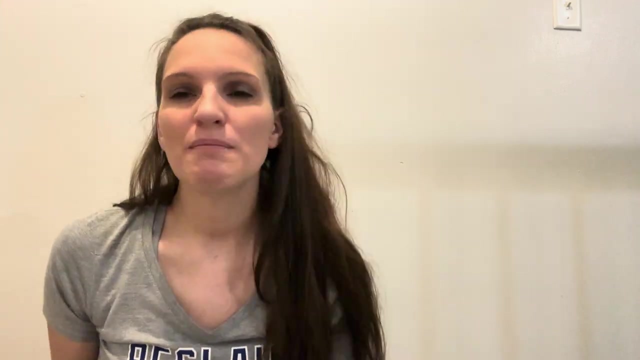 binder. so if they needed refreshing on- okay, what's a noun or what you know what's about, or whatever it is- those are kind of just notes that you can rip out of the back of the book. okay, so now language five. we're gonna kind of look over that. it is pretty much the same exact layout, um you. 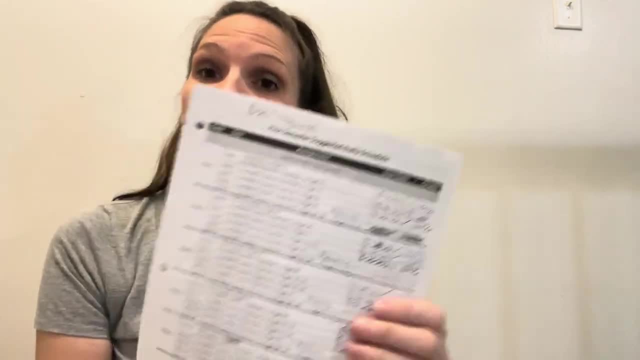 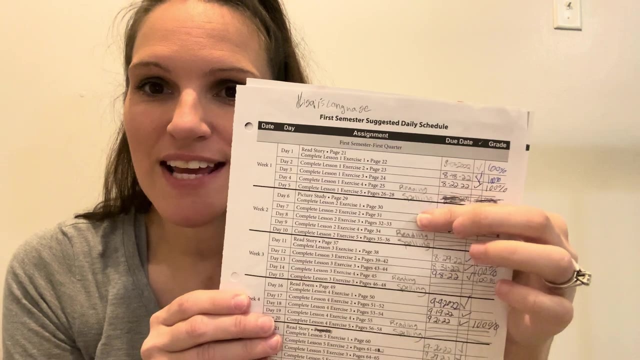 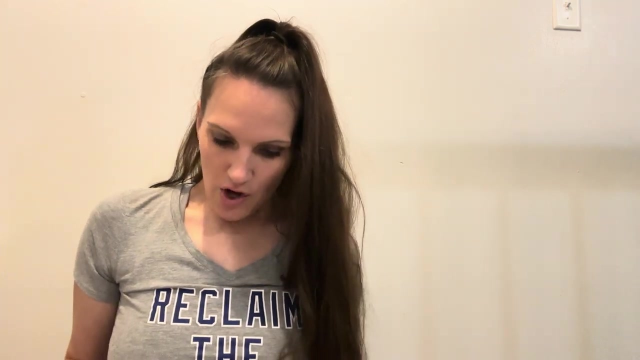 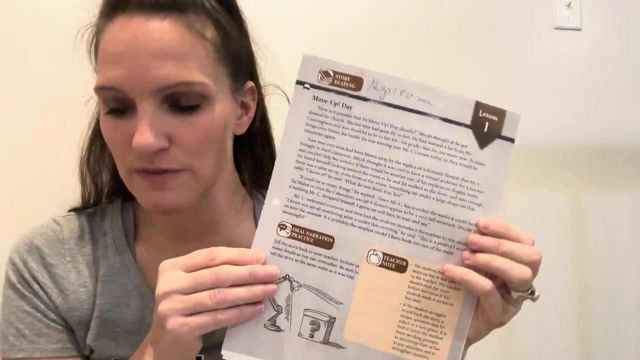 will have at the beginning of the book. you will have your plans, as i stated. you will see, as i have marked day four, students reading. day five is spelling- same exact type thing. so, um, you will be going over usually the first day, so let me pull up some of these pages. um, so it says lesson one. you'll have some reading, um, if 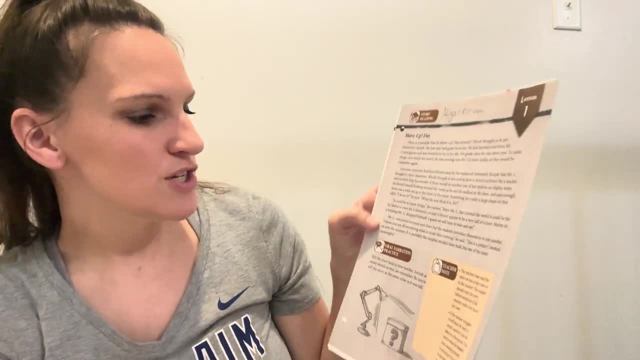 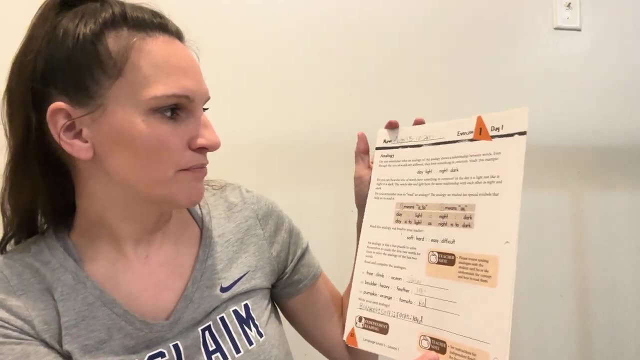 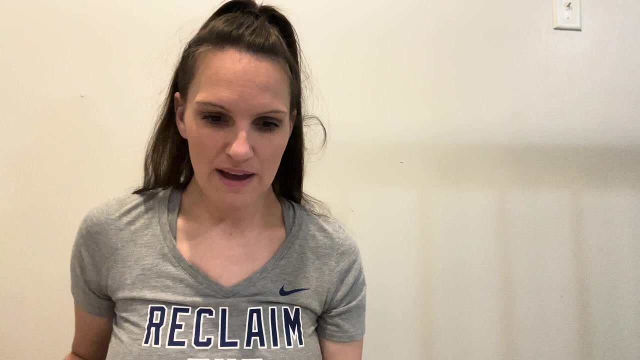 it's a picture study or or a poem. um, sometimes it's just a reading and a comprehension type deal, and this is also day one, going over some different things, and then, um, it's pretty easy about two pages a day, front and back there. so day two, you got some studying going on. 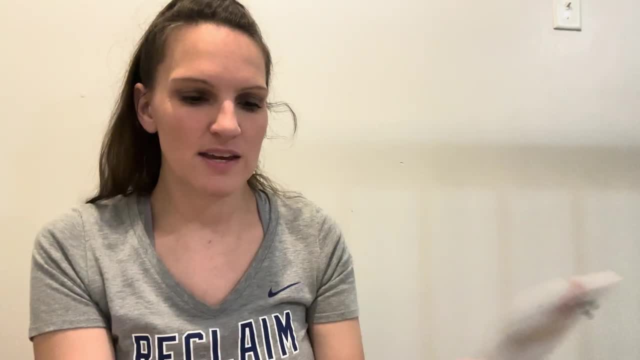 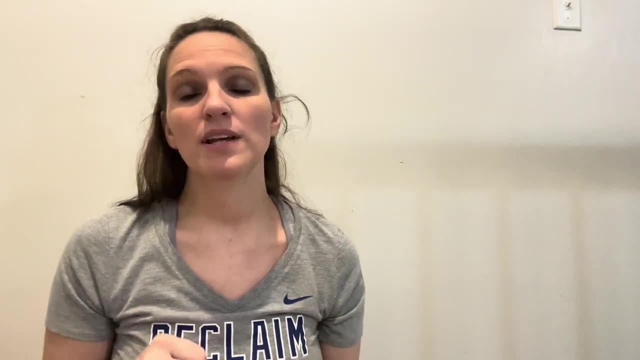 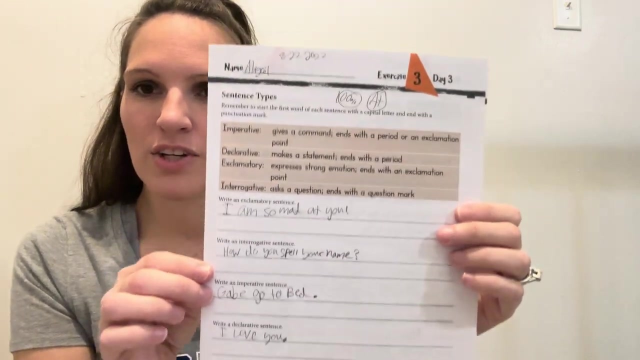 let's see grammars, nouns and different things. so you got one page on day two that week. um, usually you get about two pages. maybe one day a week you'll get one page, um. so. and then day three, you got more, more studying and learning different things, and then you got. 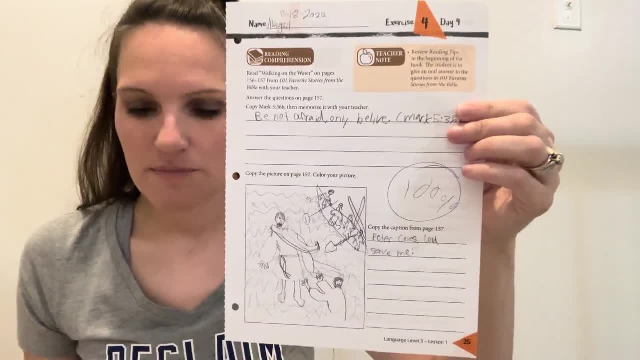 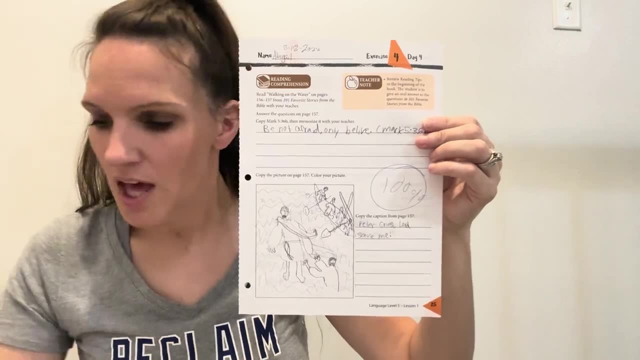 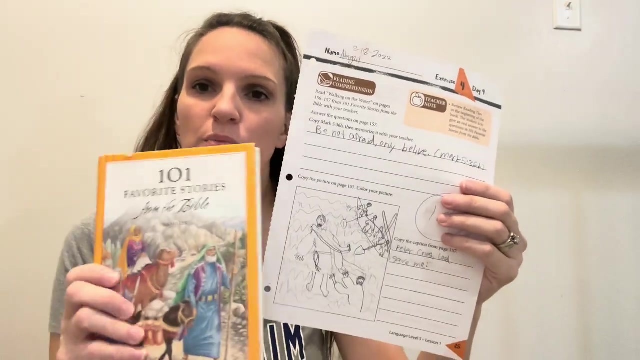 your day four, which is your bible page. um. so the thing about, um, i think, three, four and five, i'm not sure anything under grade three if you will have a different book or not. but for your day four, you will be doing this right here, so you'll be using this book also. so the same book. so i only got one. 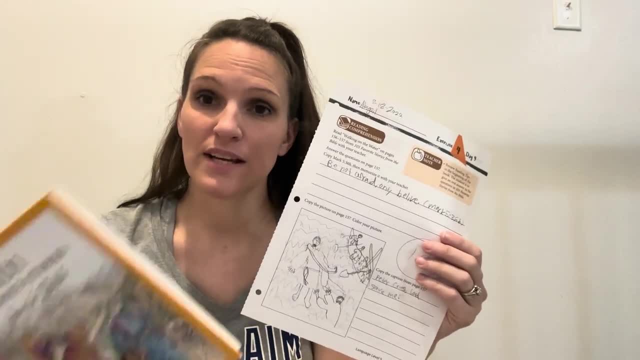 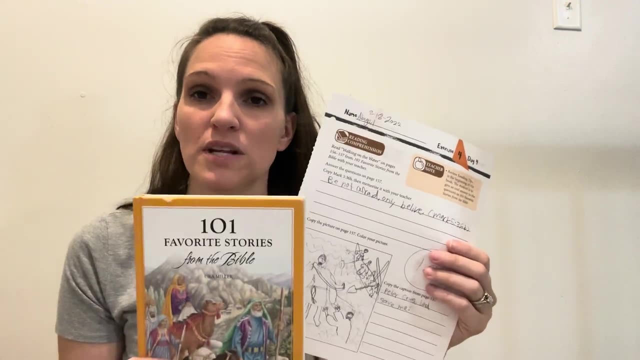 book. um, my kids could share this book. when anyone was doing it, they could do it, and then they wait until the other one's done and do it, or they could be doing a different subject or whatever, and while the other one's doing it. so there is not really a reason to buy more than one book. 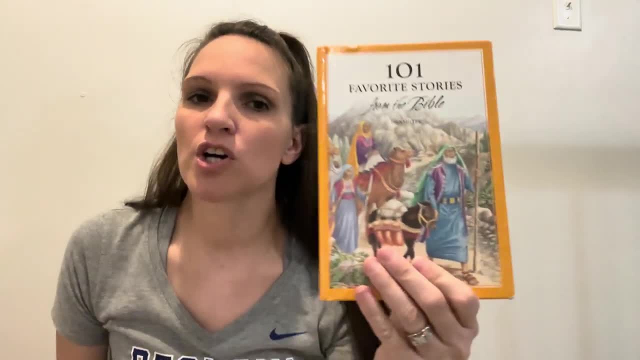 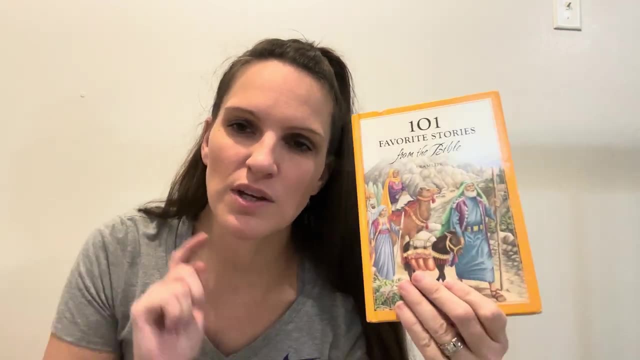 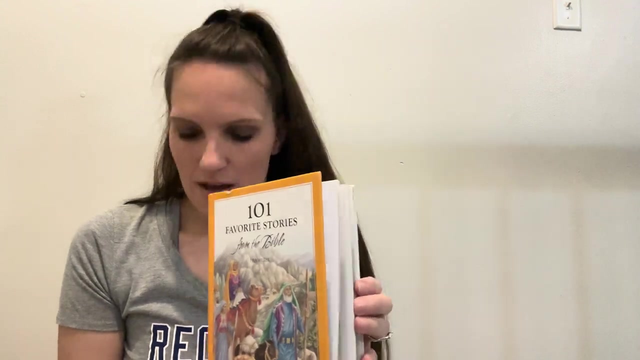 um, you have to put this in your cart. as far as i can remember, you would have to put this in your cart separately, um, or you can. if it does come with it, you can elect not to get this and not to pay the extra money. so my both of my kids, i, needed this book. um, i think some of the stories. 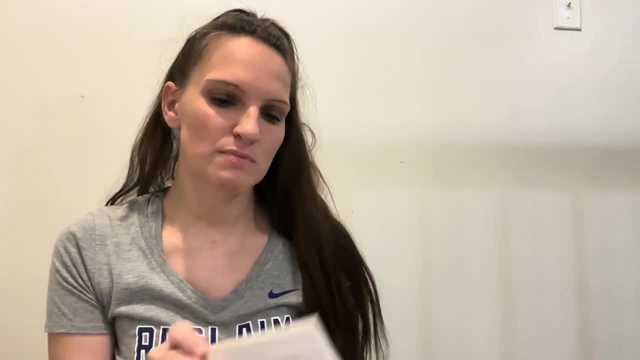 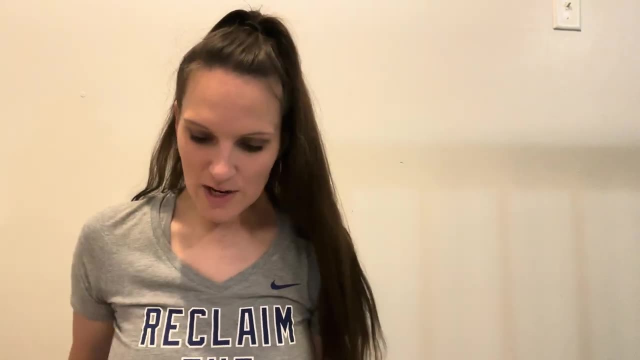 that they chose for the older would have been longer stories, maybe a little bit more difficult, um, for, uh, my older daughter, she was a couple years older than the other, so, anyways, they make it a little bit, you know, more age appropriate for the those days. so anyway, so day four you got. 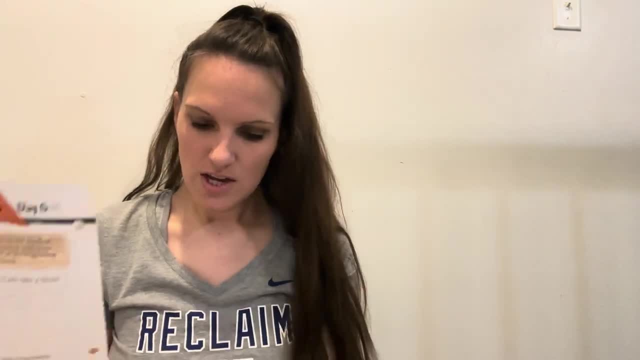 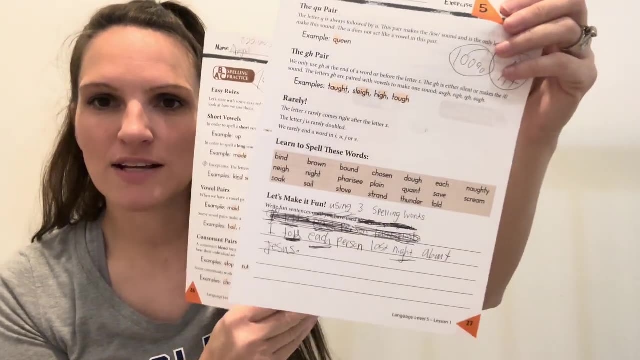 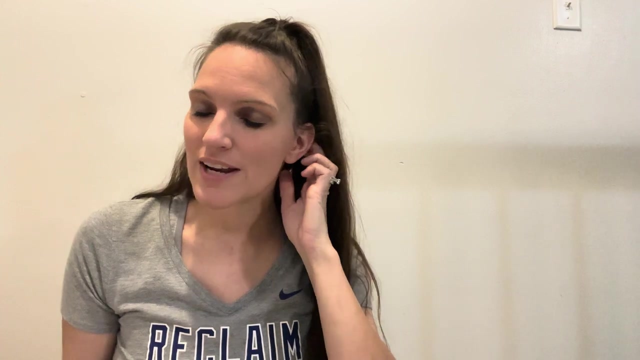 your bible. you do that. and then day five: she had some spelling going over, some spelling stuff and spelling words for day five, so she would have to do whatever that is for that one day. and, as i said, I pulled out day four reading and that was a Monday, and we pulled out day five, a spelling. 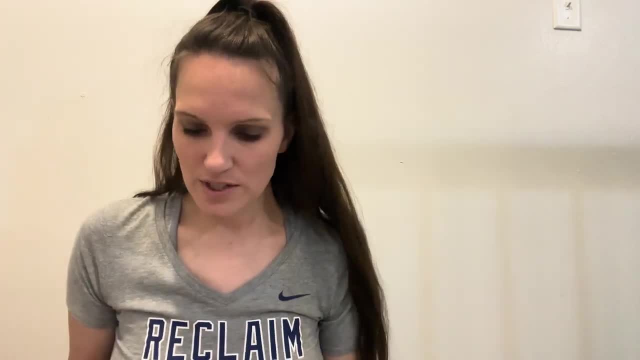 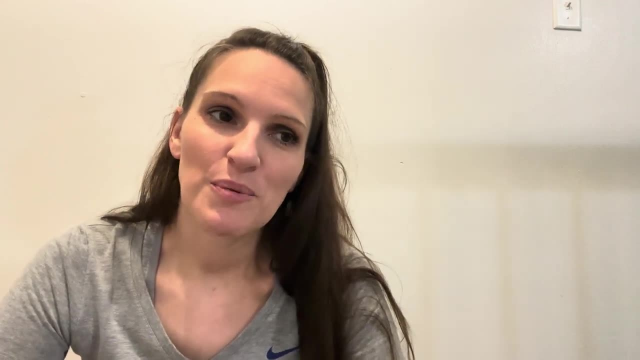 and that we use that as a Monday and then the rest of the week I had them reading different books, um, and then um spelling. I had them writing those words, which got really old. so we just got a notebook and they just had to write it and they did not like that, they just got really old. so 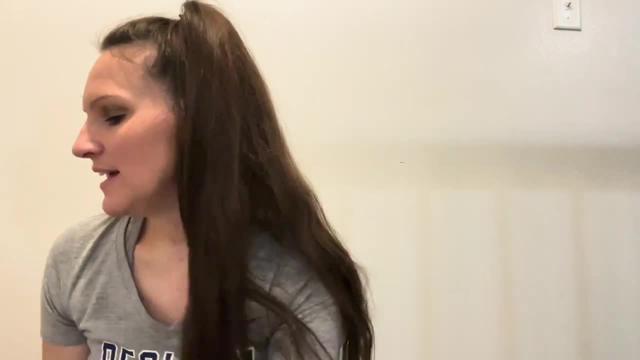 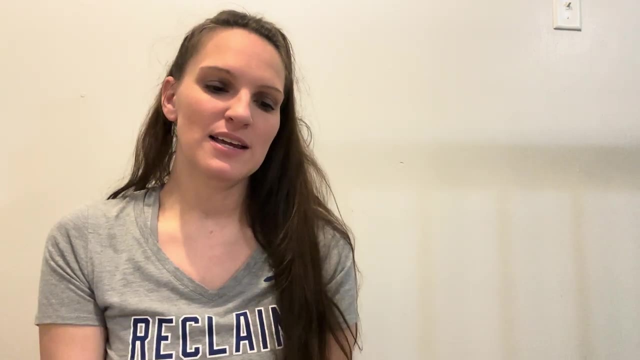 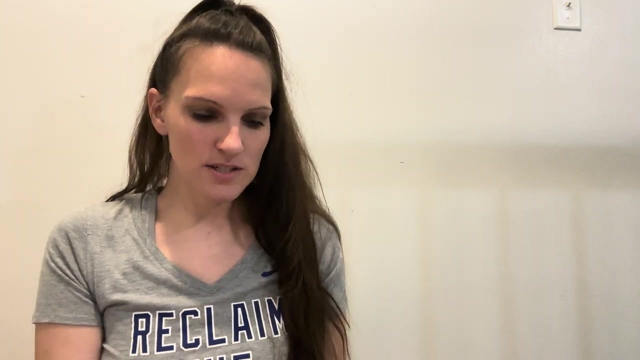 anyways. so this year we were doing spectrum, um, and then, so sorry, a lot of the pages are ripped out because she's done them. so this is what it looks like: um, again, in the beginning it has the schedule laid out and then, um, in the back it has the answers. let's see here, let's see all your. 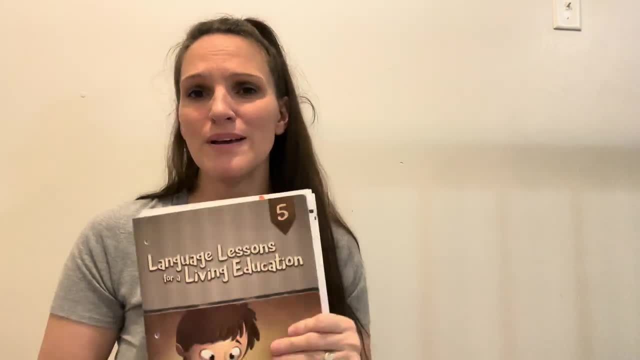 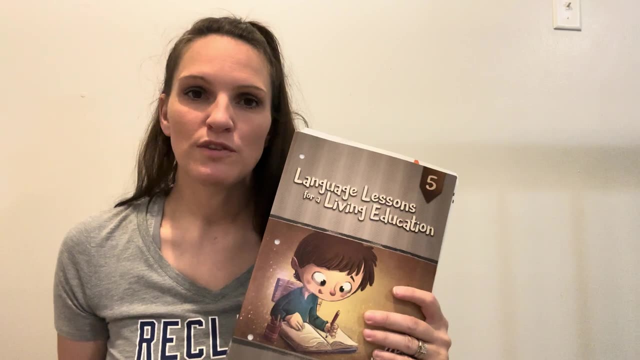 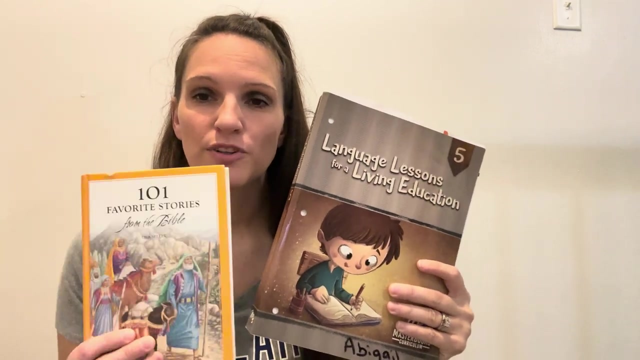 answers in the back. it's pretty similar, basically, to the other grades: same layout, type, um. so you will have same day: one, two, three, four and five, um, it'll just be different things that you're learning at a higher level. so, and you will need this book for day four if you want to do the reading. so, um, you will need. 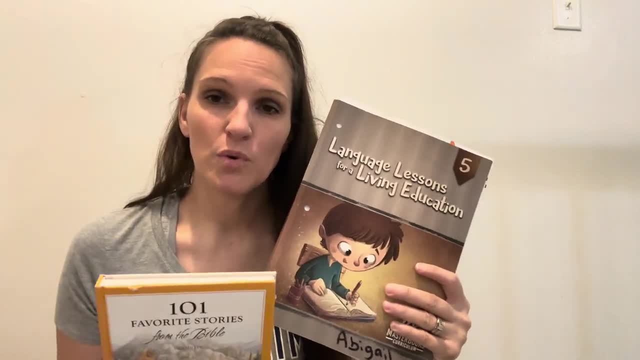 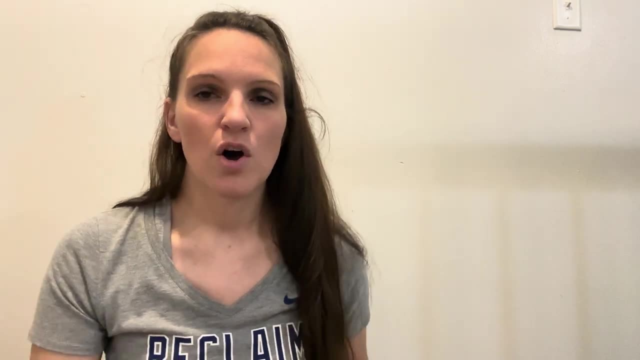 this same book for grade three and grade five and I'm sure you'll need it for grade four, um. grade six is where it changes. um, I will be doing a separate video on that. my daughter did grade six last year, so all these are last year for my kids, kids, um. so I will be doing a separate video review.